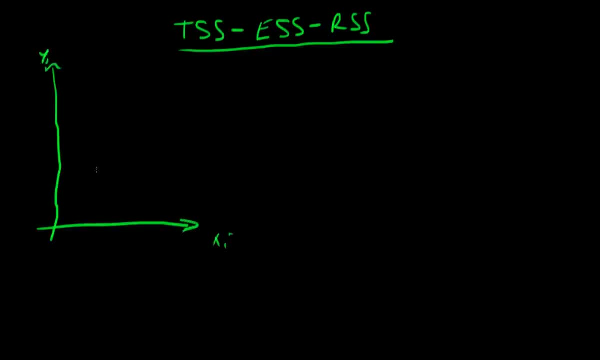 two variables, xi and yi, where yi is the sort of thing that we are trying to explain with our model. So perhaps we have some sort of data which looks something like this and we can think about our yi as having some sort of mean right. So we just calculate the mean for the yi, which is we call y. 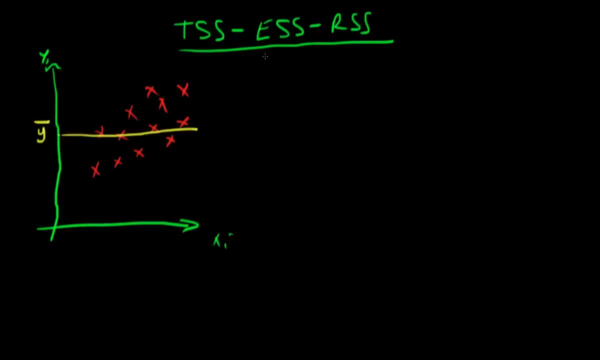 bar. We can think about the total amount of variance in our dependent variable that we're trying to explain as being the sort of sum of all the distances of points or the vertical distances of points from y bar, When, in fact, because we're going to have consider some points which are 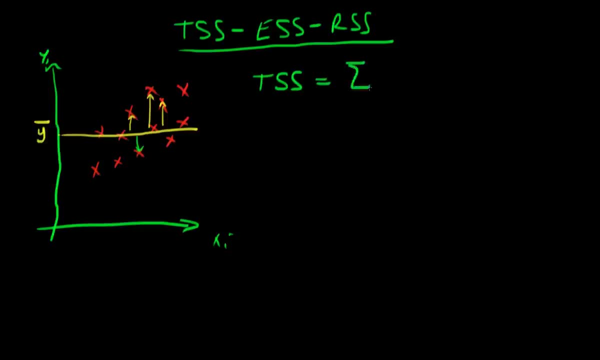 actually below the line. instead of just summing the distances, we're actually going to sum the square of the distances. So that's the sum from i equals one to n of yi minus y bar all squared. So this kind of represents the amount of variance in our dependent variable, which we're trying to 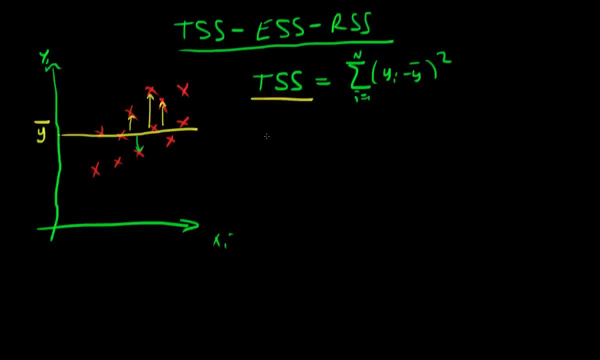 explain. So the total sum of squares is kind of the thing which we're trying to explain in our model. We're trying to explain why it is the case that our dependent variable y varies. So we might think about fitting a sort of linear model to our data. 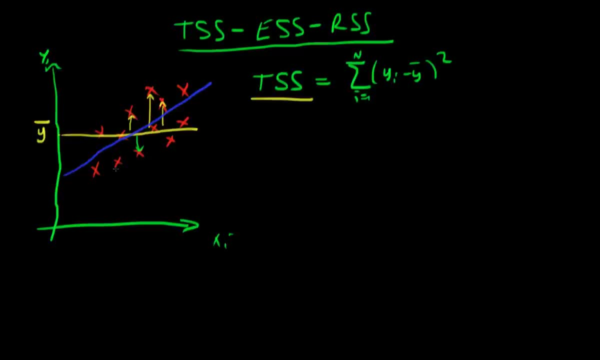 in which case we might fit, using least squares, a line that looks something like that: And for each value of xi, our model suggests a value of yi which isn't identical to the value of yi which we have in our sample. It's the serial goal, And so that's kind of the thing that we're. 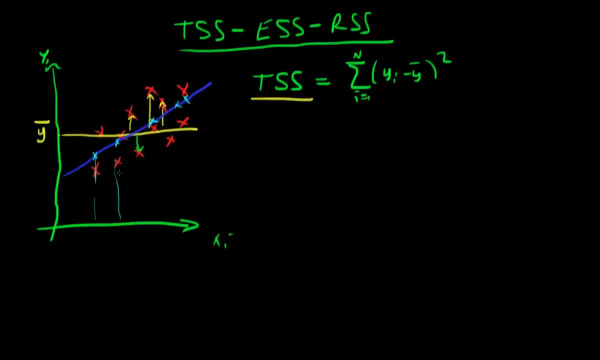 of points which lie on our line, and we could do that for each of the points in our sample. Then it might be interesting to say well, using our model, how much of this sort of variation of y or the points y from our sort of their average y bar is explained by our model, and we could do. 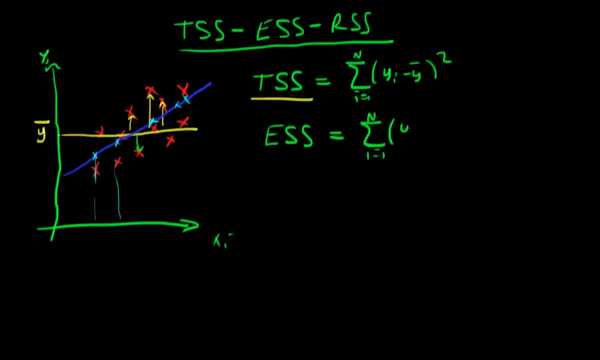 that by sort of summing up from i equal 1 to n, our predicted values of y, i minus y bar all squared. So this is what we call the explained sum of squares, because this is the amount of variation in y which our model explains. In reality, it's not frequently the case that the explained sum